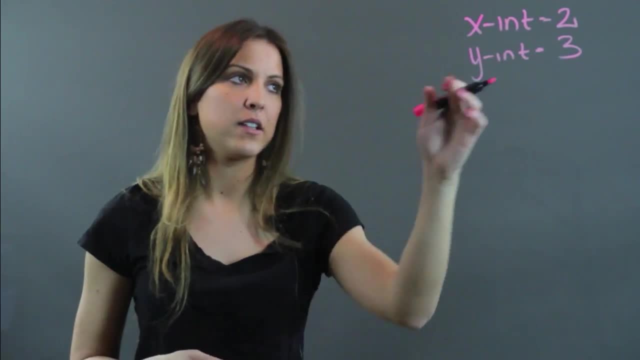 so I'm going to use that information to find the slope and I also need to find, well, the y-intercept which is given to me. So the slope-intercept form of a line is: y equals mx plus b, and these are the. 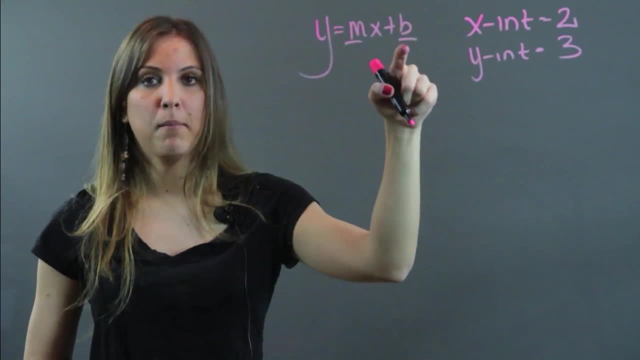 two things. I need to fill in m- my slope, and b- my y-intercept. So that part is done. I already have my y-intercept. Now to find your slope. here's what you need to do. Remember that m is always. 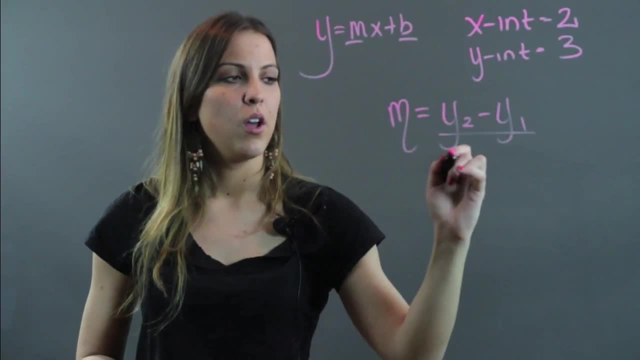 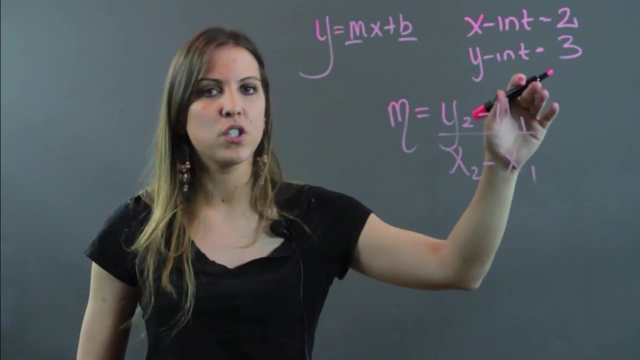 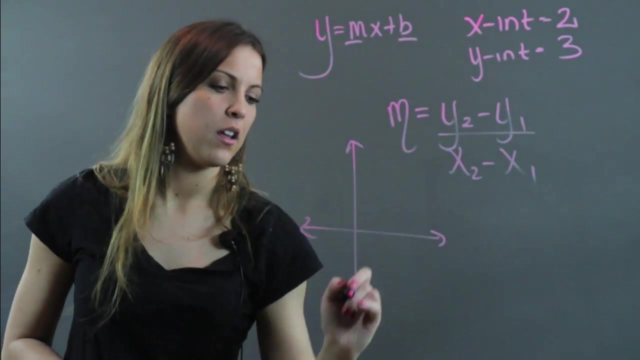 equal to y2 minus y1 over x2 minus x1.. So to find the slope I just need two ordered pairs. and with these intercepts- I'm given two ordered pairs- The x-intercept is 2.. That means, let's picture that On a coordinate plane, if my line hits the x-axis at 2, then that point. 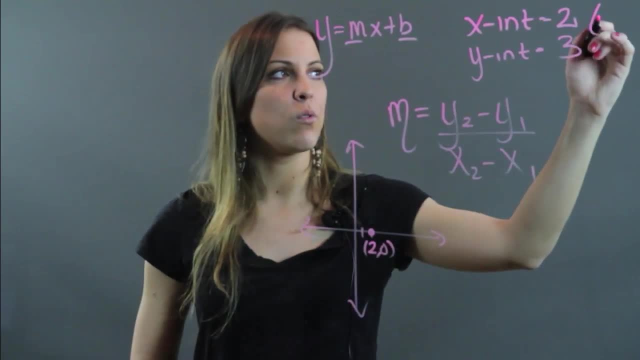 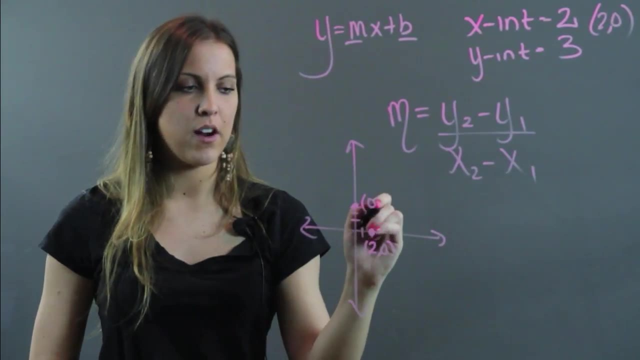 is 2, 0, right, So that means that that's actually the ordered pair: 2, 0.. And for my y-intercept, if it hits the y-axis at 3, well, the x-coordinate there is going to be 0, because that's 0, 3.. 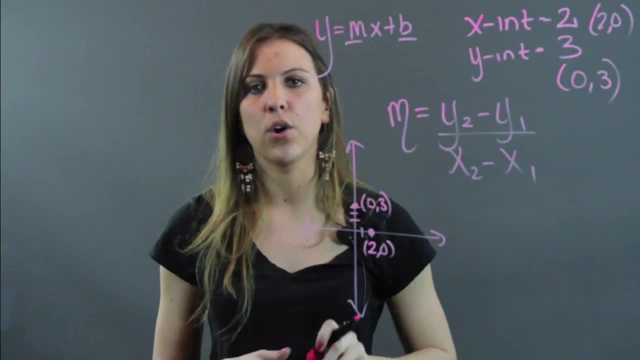 So now I do have two points. I have 0, 3, and I have 2, 0.. I'm going to use these two points to substitute into my slope equation. So I'm going to call 2, 0, my first ordered pair. 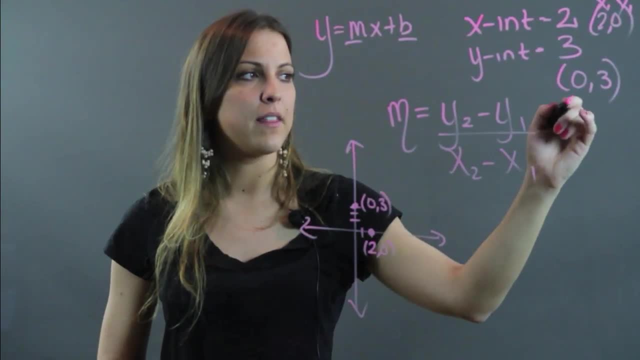 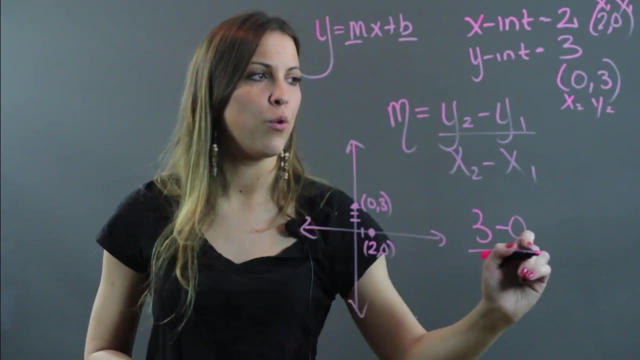 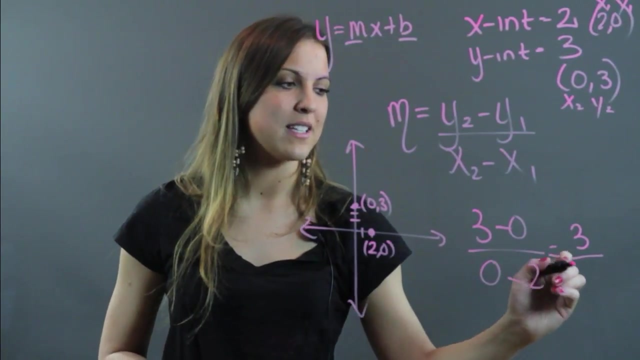 so I'm going to label that x1, y1, and then that'll make this x2, y2.. And now we're just substituting So y2 minus y1 over x2 minus x1.. I get 3 minus 0 is 3.. I get: 0 minus 2 is negative. 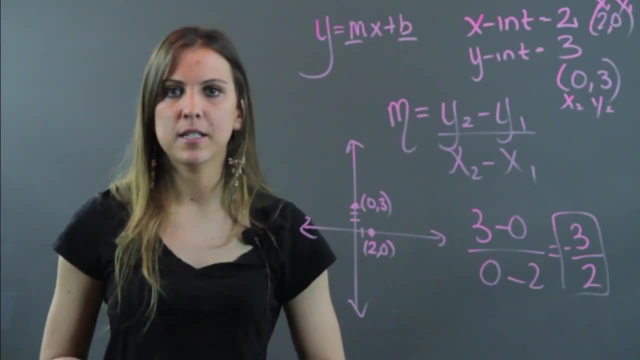 2, so that becomes negative 3 halves. So negative 3 halves is my slope, 3 is my y-intercept, and those are the only two things that I need to write the equation of a line. So it's going to be y. 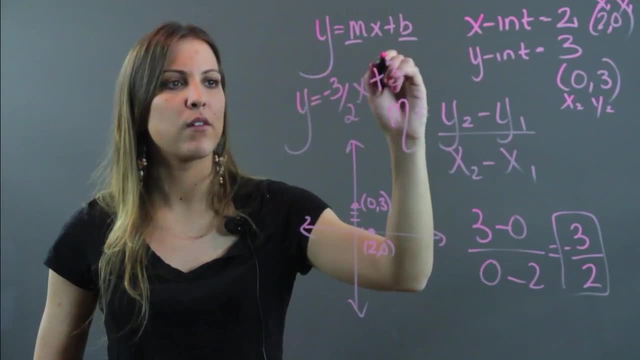 x and then my y-intercept was a positive 3, so I'm going to write plus 3, and that becomes the equation of my line. My name is Maria and I just showed you how to write the equation of a line. when you are given the x and y-intercepts but not the slope.